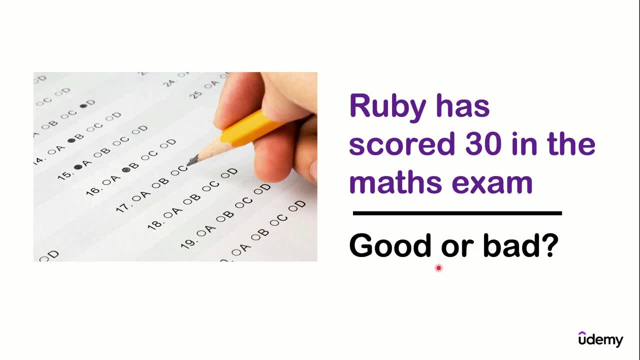 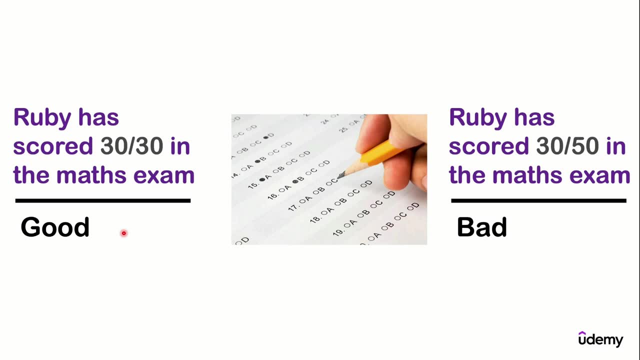 score or a bad score? Yes, no, maybe, If we don't have rightly identified. we need a base to compare or judge the performance of Ruby, right? So if it was like a 30 out of 30, it's a good score, But if it was like a 30 out of a 50,. 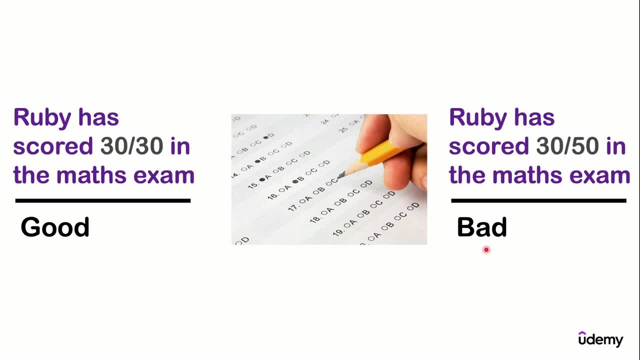 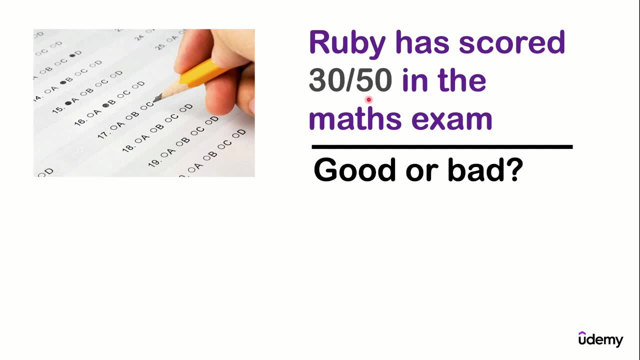 is it a bad score? Well, we can't entirely say that, right, And let's understand. why is that? See, even if it's a score of 30 out of 50,, we cannot say whether it's a good score or a bad. 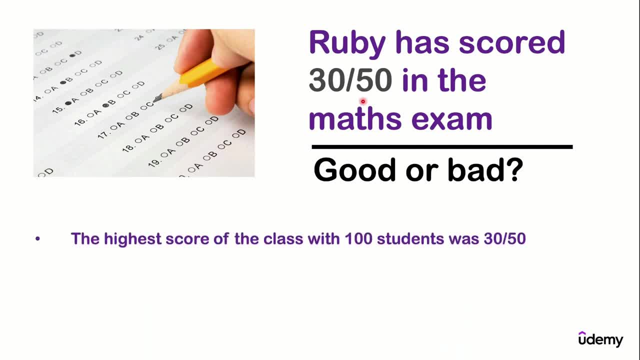 score. If you see this statement, which is the highest score, of the best score in the world, the highest score of the class with 100 students was 30 out of 50, then Ruby's score is a fabulous score. right, Ruby has stopped in the class. However, if we have this data point, which is: 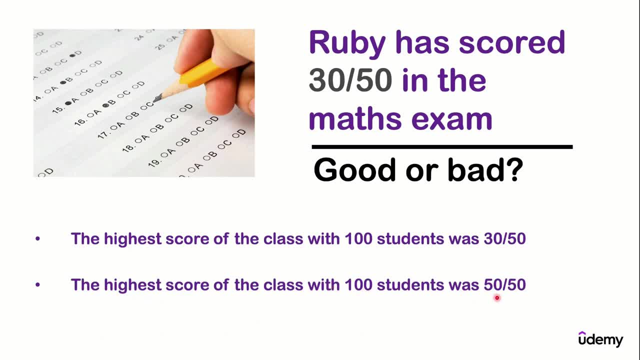 the highest score of the class with 100 students was 50 out of 50, then we can surely say that the score of Ruby is a bad score. See, the whole point of this exercise is to help you understand that, to infer if something is good or bad, or if something is high or low. 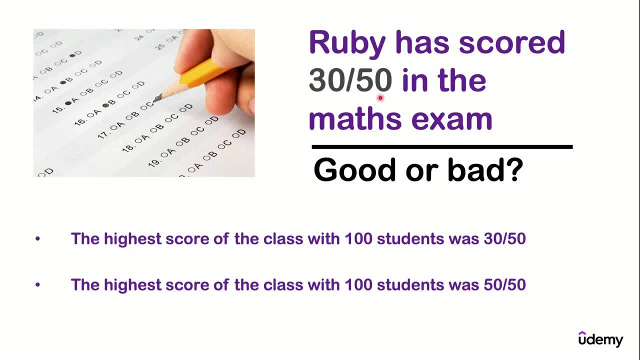 we need a base to compare. right, This 50 as a base here, or these two statements, provides a measure or a baseline to evaluate the performance of Ruby. okay, So I hope you understand that. So the learning is to compare anything. we need a base to compare and in projects, this base is. 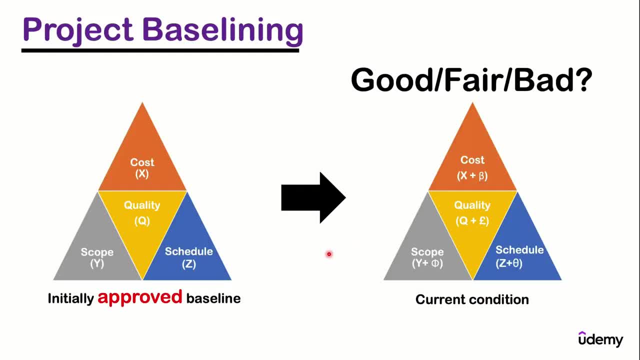 called a baseline. So what is project baselining, guys? Baselining is nothing but the initially approved scope, cost and the base of the project. So what is project baselining, guys? Baselining is the scope and schedule of a project which everyone has aligned to deliver a specific 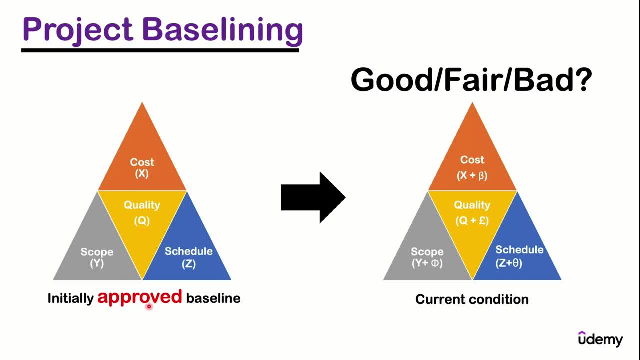 quality okay. So the red letter word here is approved. Until the scope, schedule and cost of a project is approved by your senior management, you cannot say that the project has been baselined Now. of course there can be other baselines, such as resource baseline, communication baseline. 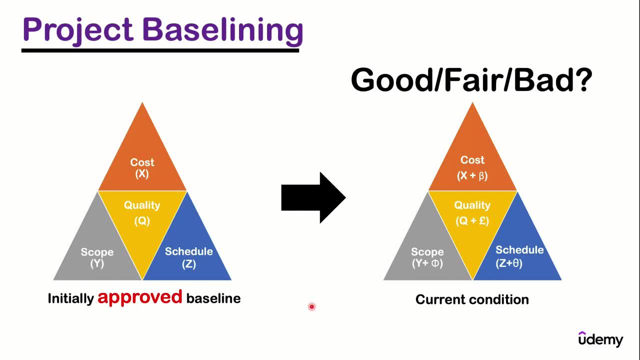 etc. But these three parameters of scope, cost and schedule are the three most critical parameters that impact the final quality or let's say, the delivery of a project. Now, in the current condition, after the project has started, if we see that x, y and z.